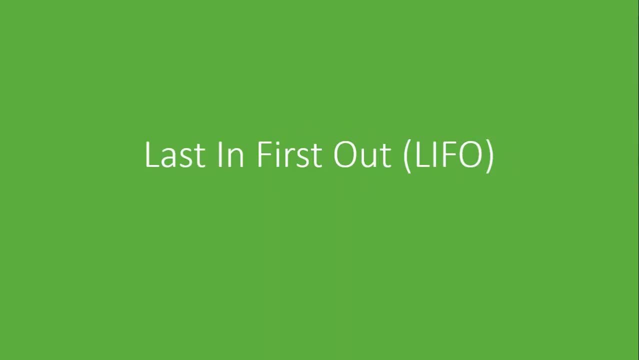 Welcome to Countouts. In this lesson we'll be looking at the last in, first out method of inventory costing. It is a costing method that is based upon the assumption that inventory or materials purchased are sold or used in the reverse order in which they are received. 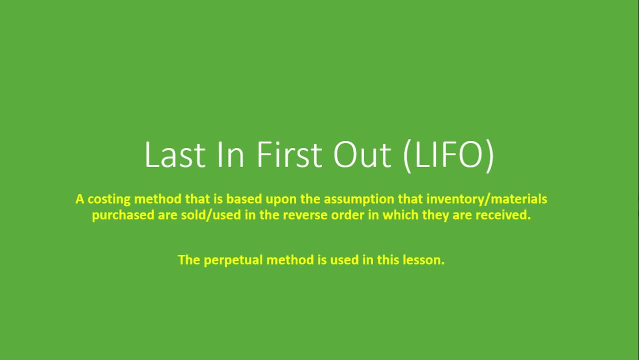 which means that the last inventory to be received will be the first one to be sold or used. We're also going to use the perpetual method, which means that we'll be updating our inventory continuously. That means that after every transaction or movement of inventory, 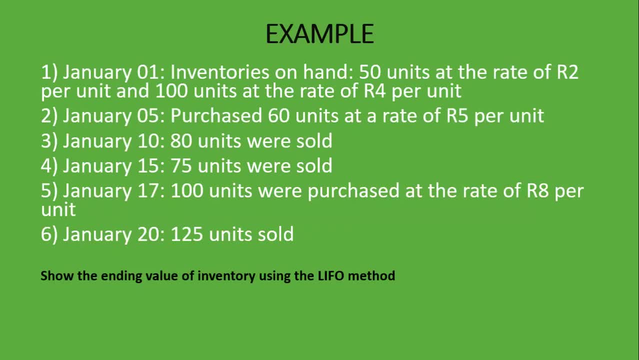 we have to update our balances. So here's an example here And we see the transactions that happened in January and it asks us to show the ending value of inventory using the last in, first out method. And here's a table that we'll be using, a very important table. 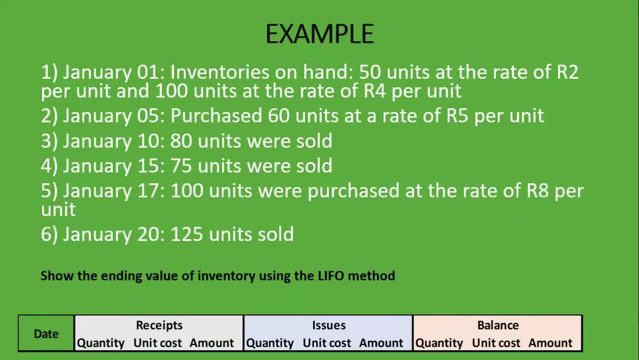 and a good table to draw. So we have date, receipts, issues and balances And under each we have quantity, unit, cost and amount. This is a very good table that will help you simplify your work and be able to document your work. 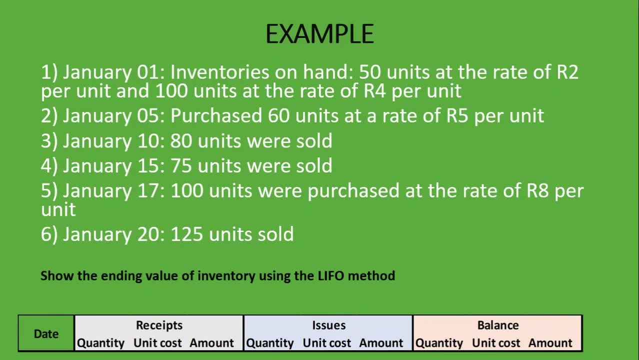 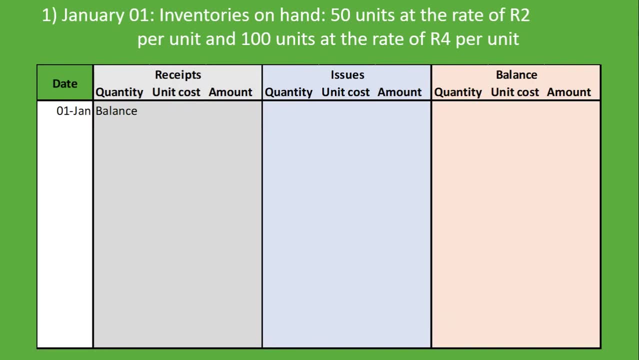 So let's look at them. The first one says that on the 1st of January, inventories on hand were 50 units at the rate of 2 rand per unit and 100 units at the rate of 4 rand per unit. So we put our date- very important to always put your date And then under receipts. 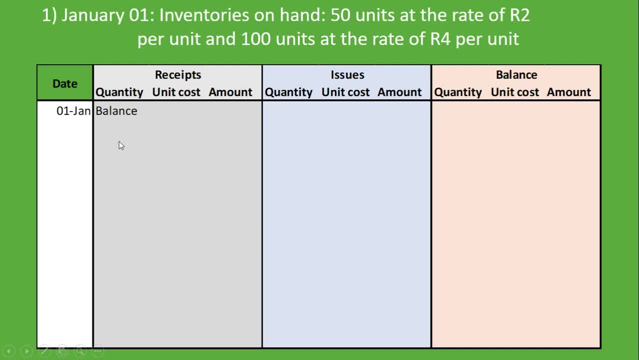 we have balances here because we are just documenting the balances we had from the previous period And then, under balances, that's where we document which inventory we have exactly. So we have 50 units at 2 rand per unit, We have a total day of 100 rand and 100 units at 4 rand per unit, And then we have our total. 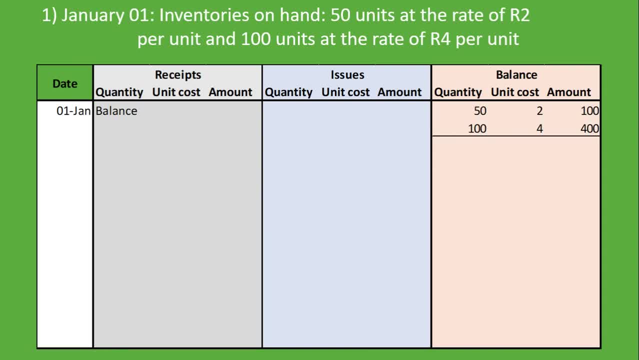 So that is how you document what you have on hand. And let's look at the second one. The second one says that on January the 5th, we purchased 60 units at 5 rand per unit, So we'll begin by putting in our date. and then we purchased inventory, So we put them. 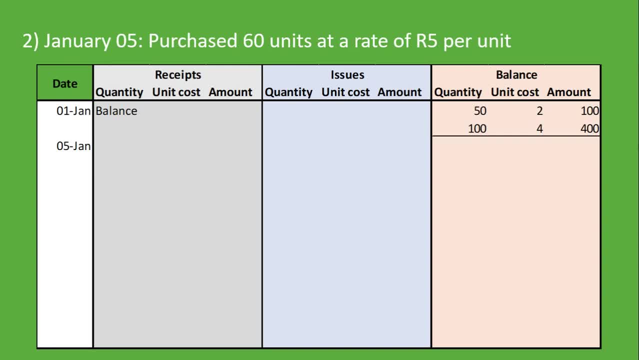 under receipts. So every time an inventory comes into our premises or our business we have to put them under receipts. So we're going to put the 60 units at 5 rand per unit And then we have our total day of 100 units at 5 rand per unit, which equals 600 rand total. 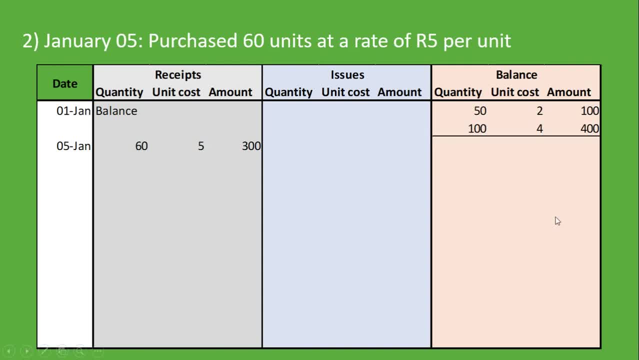 And then under balances. remember we're using the perpetual method here, So we update our inventory continuously or update our balances continuously, So we have to update all the inventory that we have in stock. So we have 50 units at 2 rand per unit, 100 units at 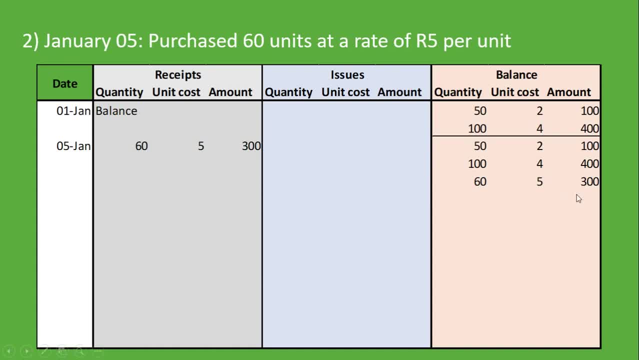 4 rand per unit And 60 units at 5 rand per unit, which we have just purchased. So there is how you should- that's what you should remember to do- always- update all your inventory And then, under balances, we have 600 units of 100 rand. This is in the 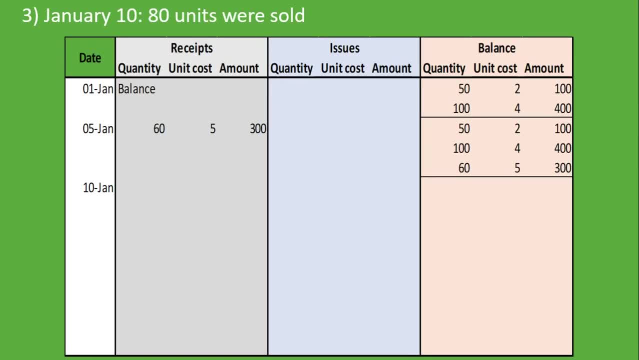 fifth one after each transaction and we are done with the second one. let's look at the third one. on the 10th of January we purchased, so we sold, 80 units of inventory. so we put them under issues because all the inventory that leaves our premises on our business will put them under issues. so we just sold eight. 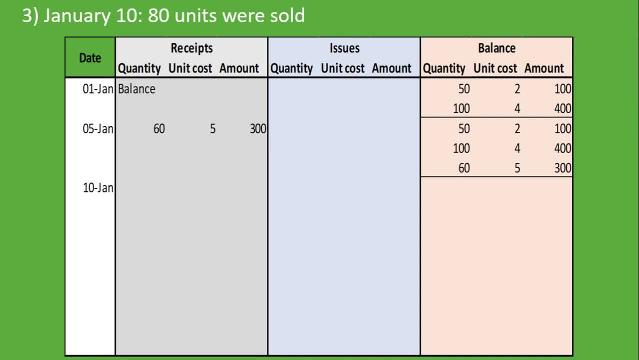 units. but remember, this is the last in, first out method. so first let's document the last inventory that we had. we haven't actually received which one was the last one that you received. we received 60 units at five and per unit. so that's the first one that will put under issues: 60 units at five rand per. 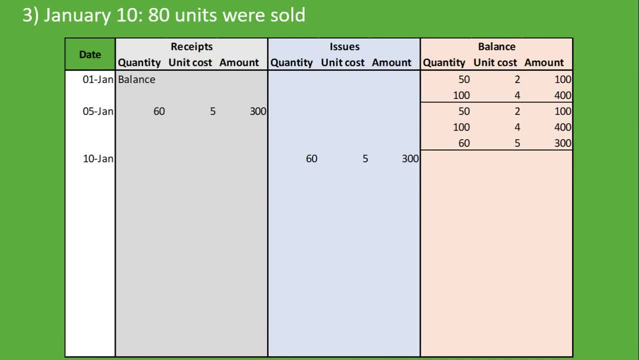 unit, but remember, we sold 80 units. so, okay, let's cancel out the 60 units. so we've just put aside all the 60 units that we last brought in. and then what is the next inventory that we brought in last? it's the hundred units that we have. 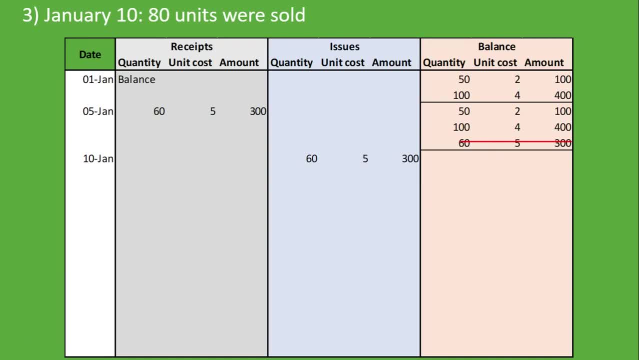 last at foreign per unit. so we sold 80 units. so we put aside 60 units. we need to put in aside 20 more units and we're going to take that from the hundred units because that's the last one we have. that's the last one that we we brought in, that we still have in stock, so we 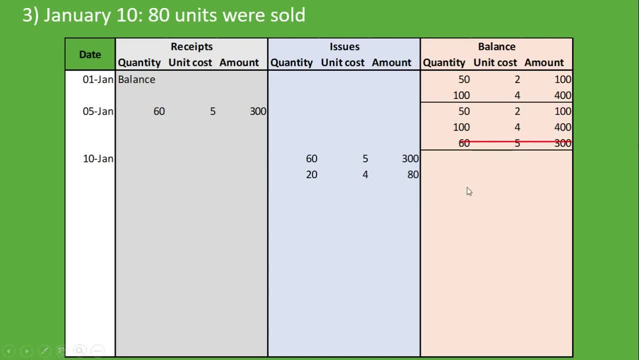 have 20 units at foreign per unit because we took them from the hundred units and that's the total of 80, 80 rand. so we have just put aside all the units. we just sold all the units that we wanted to sell, which is 80 units, and 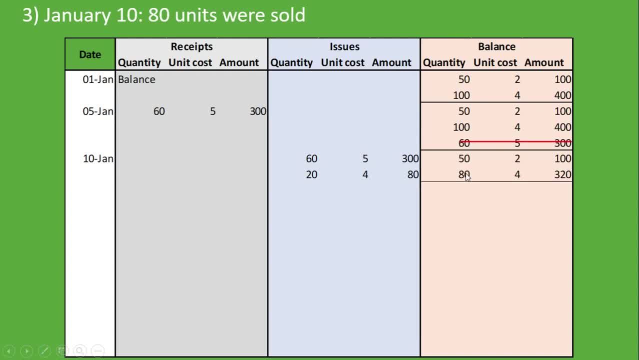 then what is our balances? we still have the 50 units at two rand per unit, and then from the hundred units, remember we took out 20 units, so we are left with 80 units at four rand per unit and we put in our totals there. so we still have the. 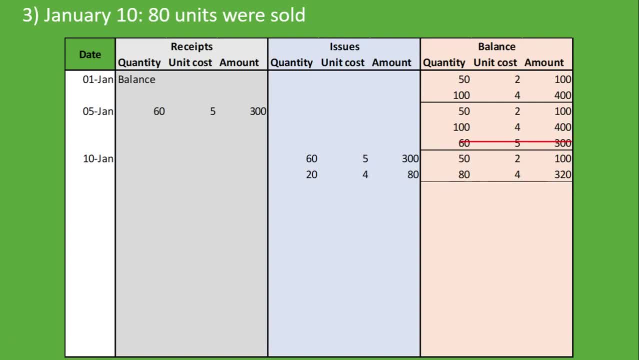 fifty units that we need to sell. so we're going to take the 80 units at four rand per unit. now that we have sold fifty units, we need to come and go and sell here all the eight units and the 25 groups, and then we press there to go out. 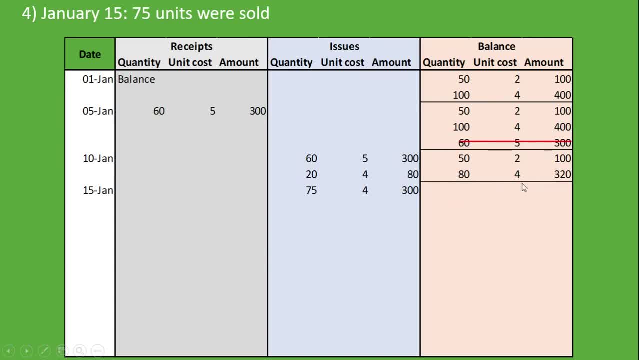 and to see all the units that we have taken, all the units where we begin. the difference of one unit we put six to the eight- I believe we have seven units- was 300 rand. and then what is our balances? we still have the 50 units at 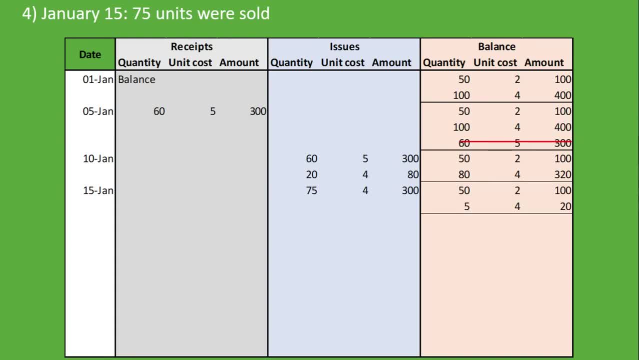 two rand per unit and then from the 80 units- remember we just sold 75 units. so 80 minus 75 gives us a balance of five rand, five units and it's at foreign per unit and we have 20 rand. so those are the units that we have in stock, the 50. 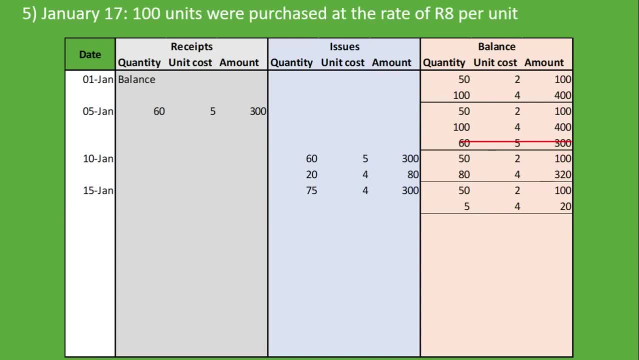 units and the five units- and let's look at the fifth- one hundred units were purchased at the rate of eight rand per unit. so we just purchased hundred units. so we put in- we're gonna put it under receipts. so we put in our date, 17 January, and under receipts we have hundred units at eight rand per unit. 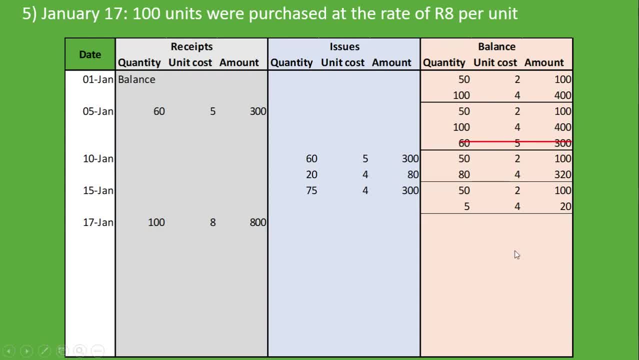 equals 800 rand. so under balances we put in all the inventory that we have in stock. so put in 50 units at two rand per unit, five units at foreign per unit and the new inventory that we have in stock, which is hundred units at eight rand per. 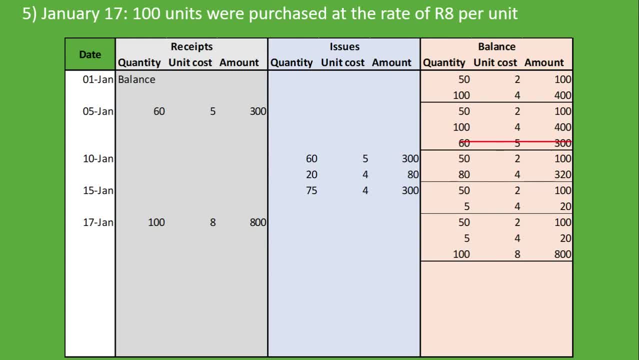 unit, and that's how is easy it is to record inventory using the last in, first out method. then let's look at the next one. January the 20th, we sold 125 units. so you can post a video here and try and and do it yourself to see if you understand how it works. and then we 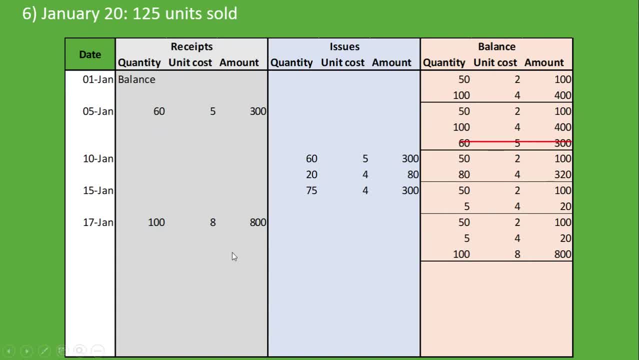 look at it. so how do we do this? one remember: we put our date 20th of January, and then how many units? as we said, we sold hundred units, so how many units do we have last? we last purchased hundred units at eight rand per unit, so that's. 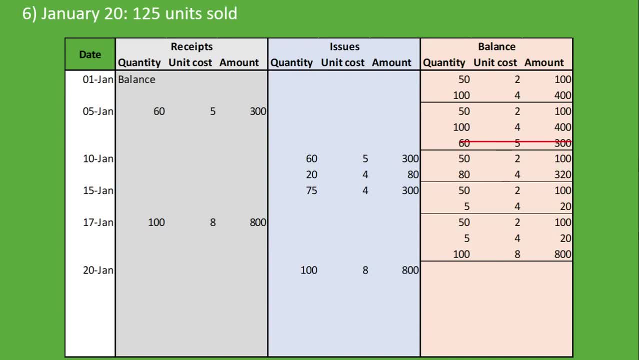 what we're going to put us in stock. so that's how easy it is to record inventory using the last in first out method. then let's look at the next one side, because we saw 125, so put in the hundred units at eight rand per unit, and 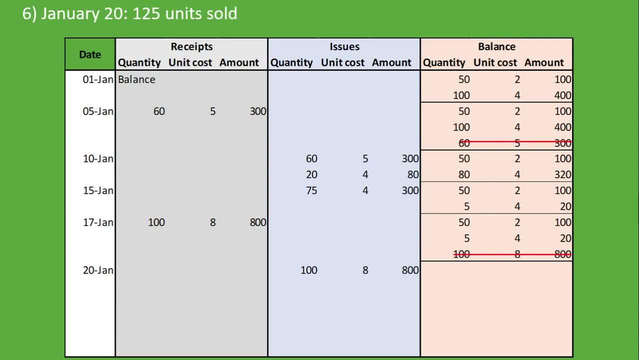 we've taken all the hundred units, so let's cancel that. we've cancelled the hundred units at eight rand per unit, and then how many more do we still need to put aside? we've just put hundred units, so we need 25 more units because we sold. 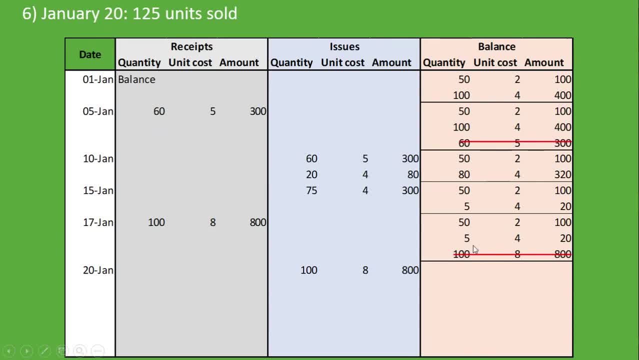 hundred and twenty five units. so we're gonna take the next one that we have that we brought in last, which is the five units at four rand per unit. so we're going to take from there five, five units at foreign per unit, and we've just taken all of them. so let's cancel that one out. and then how many do we still? 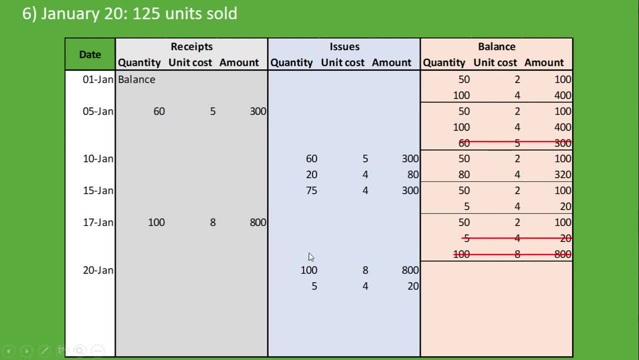 have to put aside so that we can sell the hundred and twenty five units. we have hundred plus five, which is hundred and five. so hundred and twenty five units that we need to sell, minus hundred and five that you have put aside, we have twenty more units to sell, so we're going to take them from the next batch that we 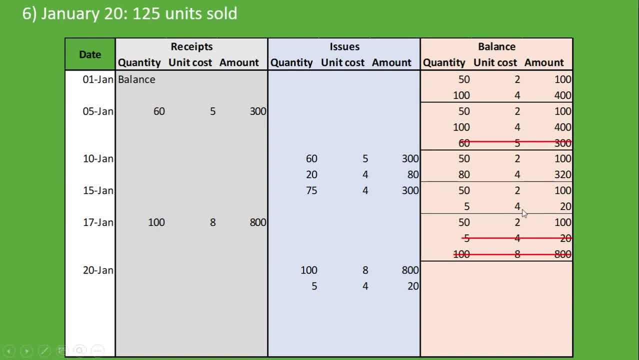 have that you brought in last, which is the fifty units at two rand per unit. so we want to take the twenty from there. so twenty at two rand per unit gives us 40 rand, and we have just sold the hundred and twenty five units. hundred plus five plus twenty units, we've just all sold. 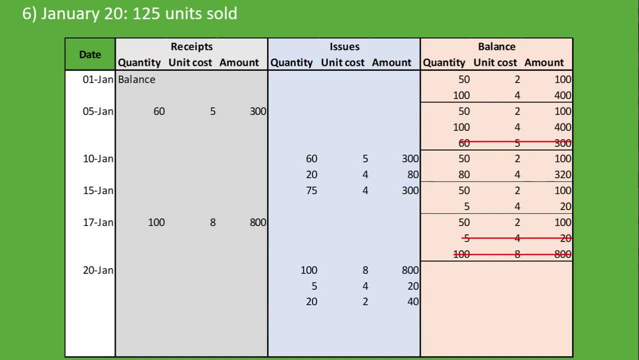 all that we needed to sell. now what? how many units do we have in stock? what is our balances? well, remember, from the fifty units at two rand per unit, we just took the twenty units, so fifty minus twenty, we have thirty units left at two rand per unit and the total is sixty rand. I hope, if you tried it, that's how. 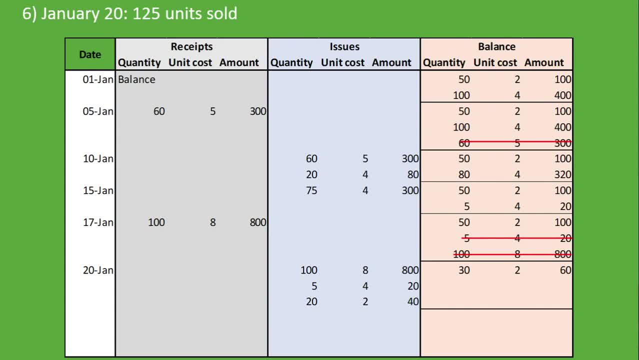 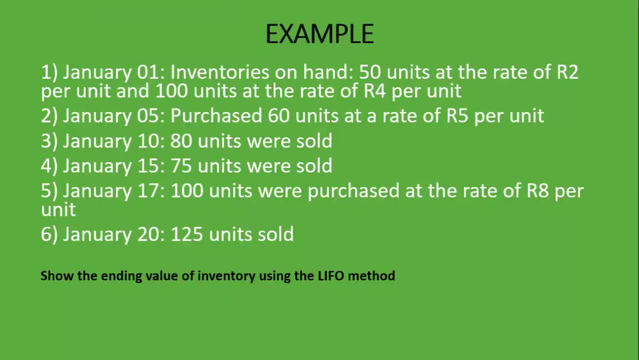 what you got and you got it correctly, and that is how simple it is to do this: to record the movement of inventory using the LIFO, and that is it. we are asked to do these six transactions and we have done them. and it asks us to show the ending value of inventory using the. 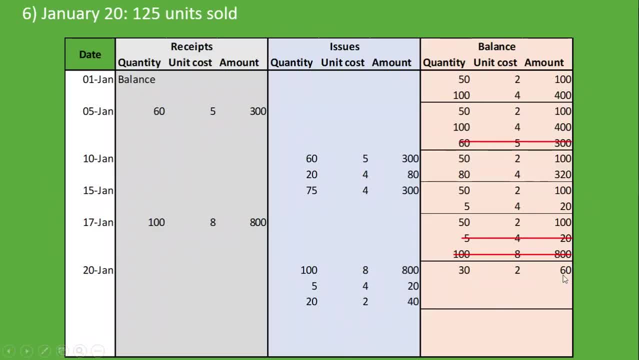 LIFO method and that's what we've just done. the ending value of inventory is 60 rand because it's thirty units at two rand per unit which were remaining and it's sixty rand. I hope that has made sense. if you have any questions or queries, leave. 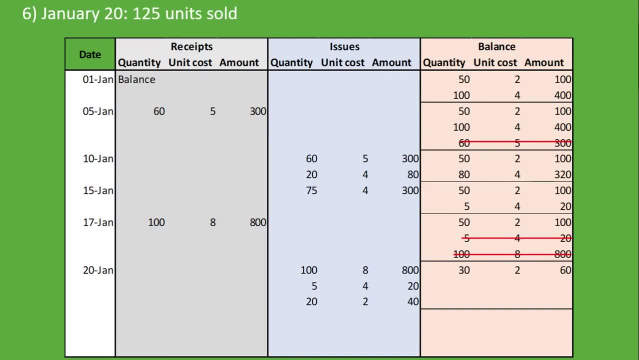 them in the comments below. otherwise, we have another tutorial using the FIFO method or the first in, first out method, which should appear on your screen right now, and if this video has helped you in any way, please consider subscribing and liking our video and sharing, if you can. till next time, cheers.